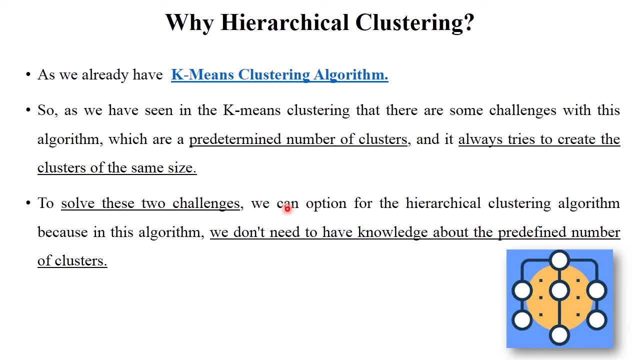 clustering algorithm. First point: no, It is based on supervised learning technique, right? second point: It has predetermined number of clusters. It means that before solving the example, you must know the how many clusters are there. So you predefined this thing, that is, K is equal to 3, like that, right? and third point: is every clusters? 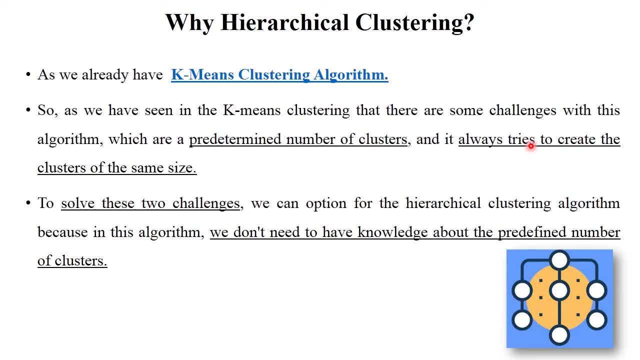 having the same size in K means clustering technique. So hierarchical clustering is just opposite of this algorithm. hierarchical clustering is solved. This two kind of challenges and this two kind of problems in this particular concept. first, it works on unlevel data set, not a level one. second, 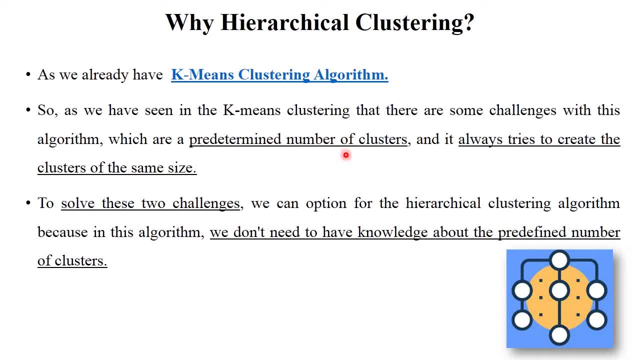 There is no need to predetermine number of clusters, right, because here we don't need to have a knowledge about the predetermine or predefined number of clusters and there is a no same size of each and every clusters, right? So that's why this hierarchical clustering work on unsupervised technique. 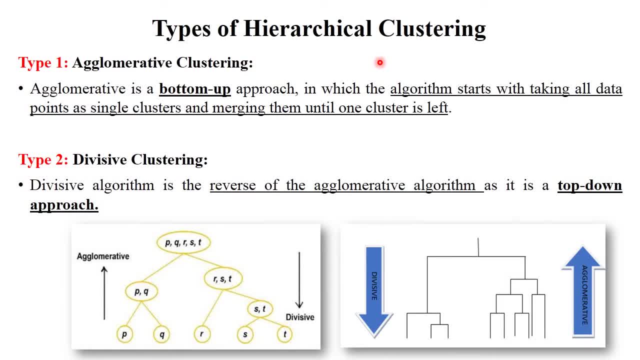 The next point is types of hierarchical clustering. There are two types. one is agglomerative clustering. second one is divisive clustering. see here in this diagram: agglomerative clustering always work from bottom to up approach and divisive clustering always work or they will perform or form the clusters in top to bottom format. 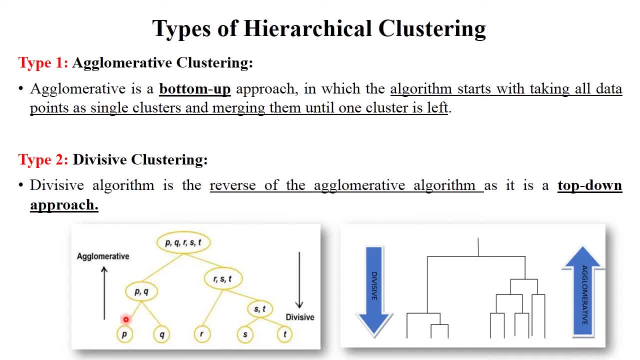 So these are the two types of clustering. now just see her in this example. first, agglomerative clustering. so agglomerative clustering always form the cluster from bottom to top. now see here there are some bottom single clusters are there like P is a single cluster, Q, R, S, T. now, so agglomerative. 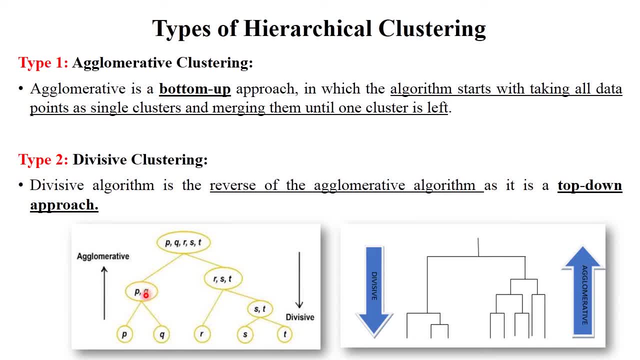 clustering, form this two cluster and made this one cluster, that is P and Q. similarly, S and T combine into ST cluster. then again R is combined with this ST and after that, at the last, this two clusters are combined with this, that is P, Q, R, S, T. 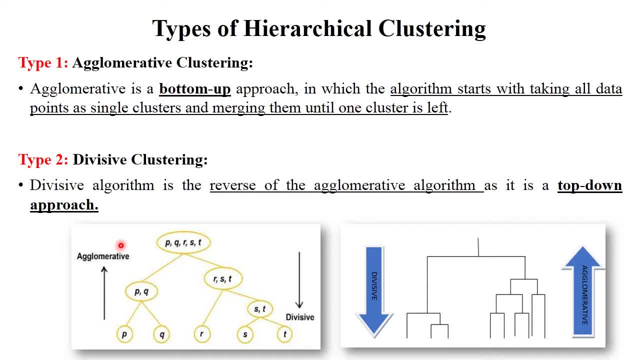 So in this way they work from bottom to top and the opposite of that. see here, that is divisive clustering. So divisive clustering work top to bottom means there is a only one cluster is there and you need to device those cluster into the single cluster or multiple clusters, right, for example, PQ, RST. 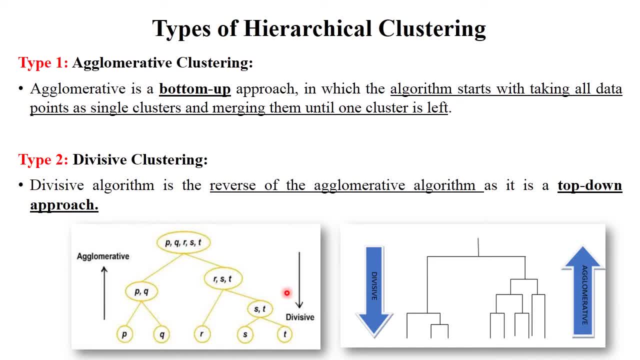 This is the one main cluster is present. So divisive clustering device dose cluster into the two parts, like PQ or RST, again those divided into the two parts ST or RST, And again this divided into the single cluster like S or T. similarly they device those cluster into the 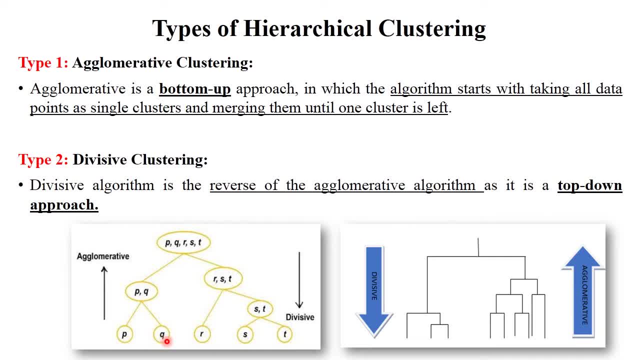 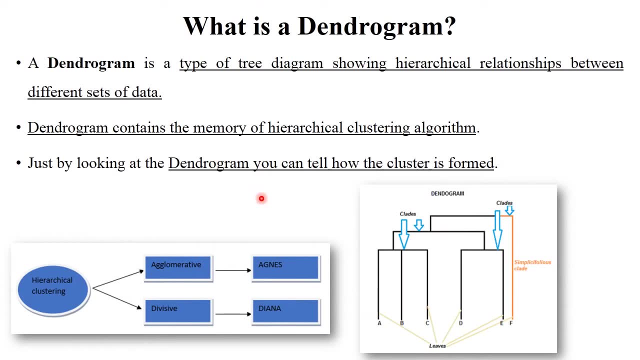 PQ, again divided into the P and Q, that is single cluster. So these two types of clustering will work as per the requirement of your project and this is a kind of type of hierarchical clustering. next, next point is: what is dendrogram? So what exactly dendrogram? so dendrogram generally used as a representation of hierarchical cluster. 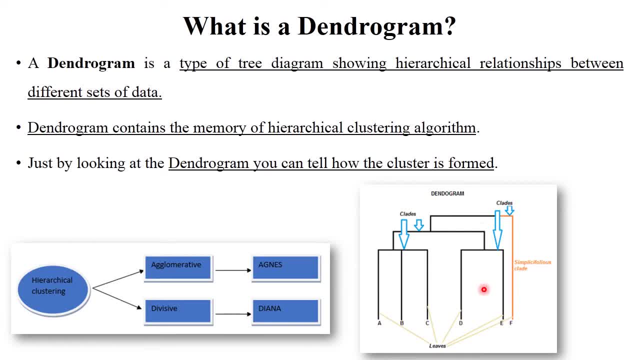 See here. this is a tree type diagram and it shows the hierarchical relationship between different data sets or different clusters, for example this ABCDEF. these are the clusters, or single clusters, or this is called as leaves, and after combining those cluster, like A, B and C, these three clusters are combined here. 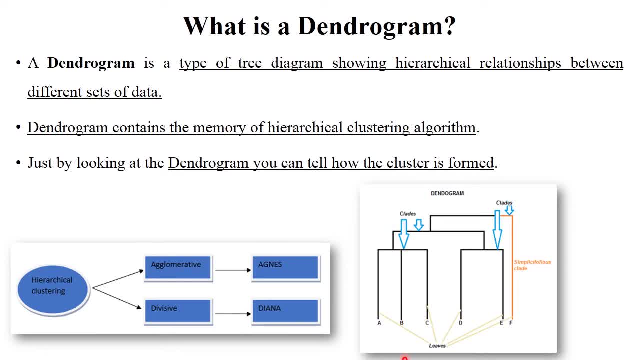 this called as clades. Okay, so in this way this clusters are represented and it's easy to find Out how many clusters are there by using this dendrogram. So this is called as dendrogram. It is a hierarchical structure. represent different clusters. 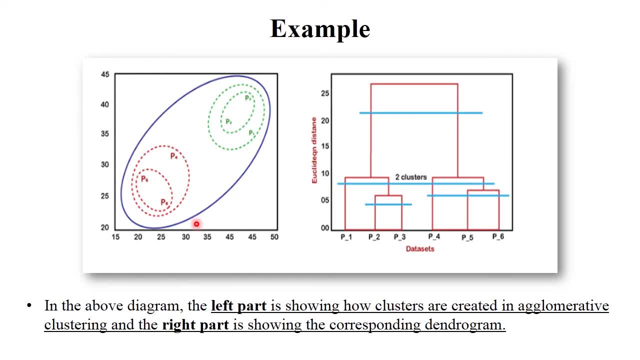 Now the next point is examples. So this is an example of hierarchical clustering, now just focused here on the left side. This is the left part. So here it represent agglomerative clustering. see, here There are different clusters are present. first, cluster P2 and P3. 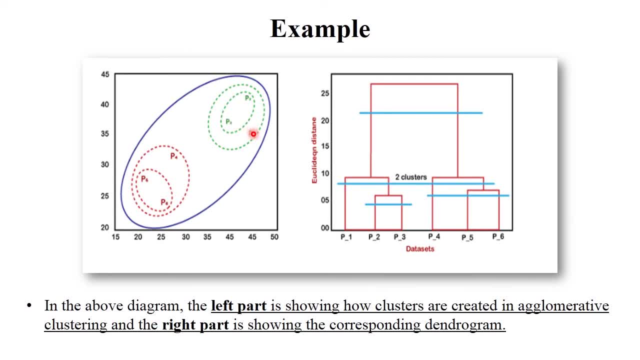 Second cluster, P1 is combined with that. that is P1, P2 and P3. right the next cluster, See here, that is a P5 and P6. after that P4, P5 and P6. This is another cluster and at the end this four cluster are combined with the one cluster or in it is in. 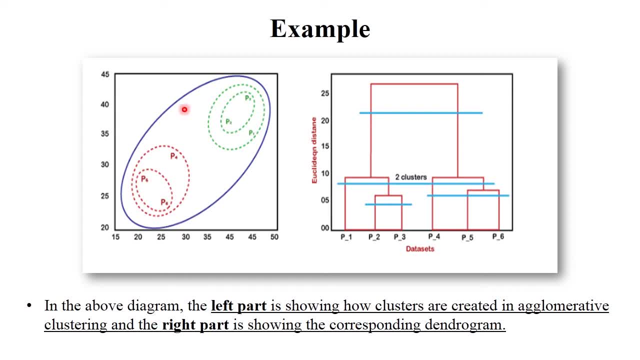 in Universal cluster, right. So now this agglomerative cluster is converted into this dendrogram format. See, this is the dendrogram structure. This is called as hierarchical Clustering. now, on the x-axis there is cluster name, or data sets are present. on the y-axis,